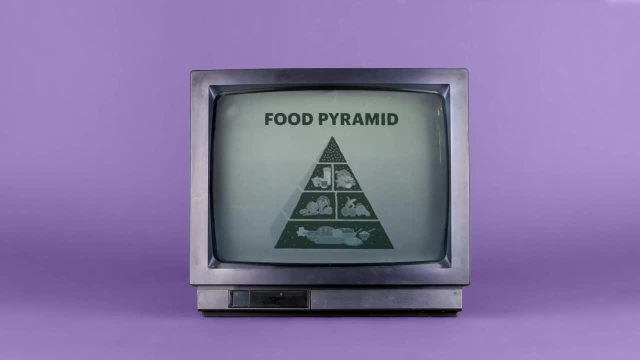 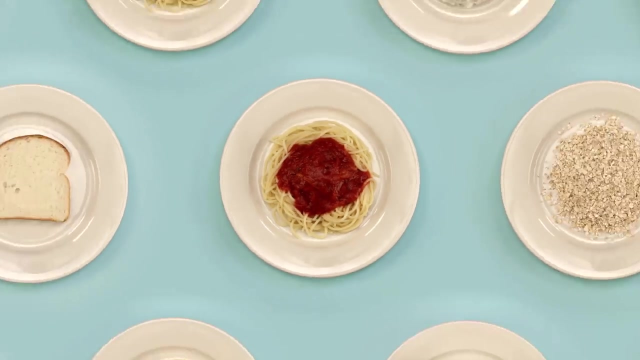 90s. kids will remember the Food Pyramid When it debuted in 1992, it was touted as sound nutritional advice grounded in the latest scientific and medical knowledge. Kids were taught they could enjoy up to 11 servings of bread, cereal, rice and pasta every day. 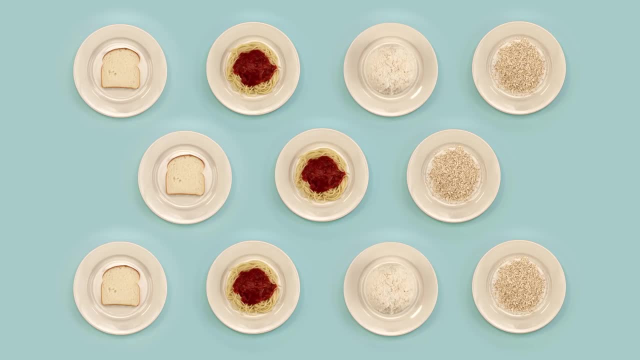 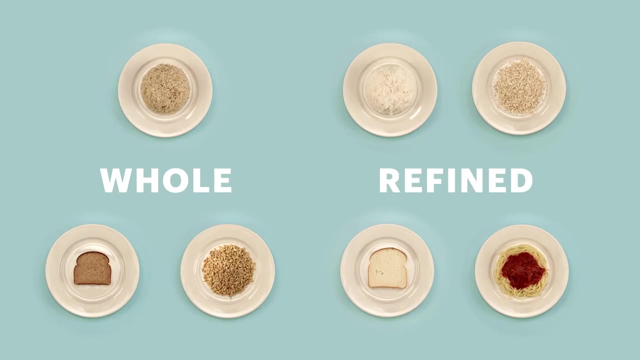 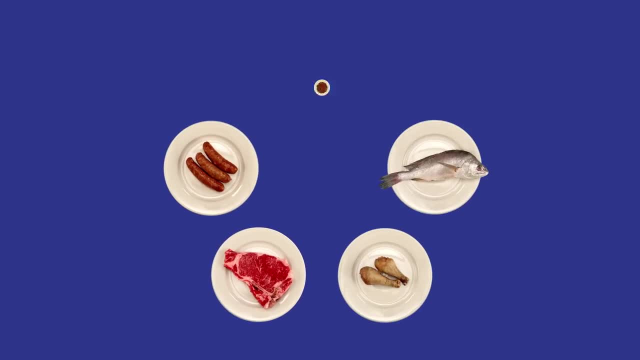 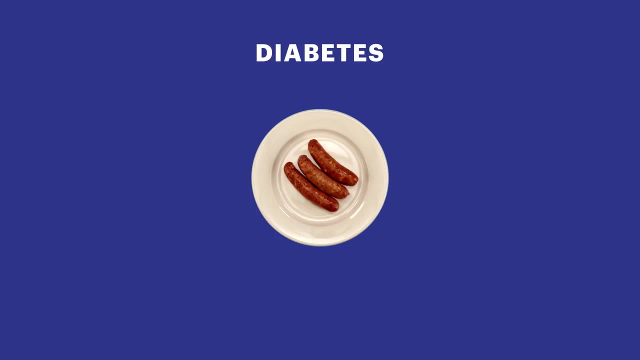 In the protein section, healthy proteins such as poultry, fish and nuts were lumped in with red and processed meat. Eating too much red meat has been linked to a higher risk of diabetes, heart disease and some cancers. Fats, oils and sweets. 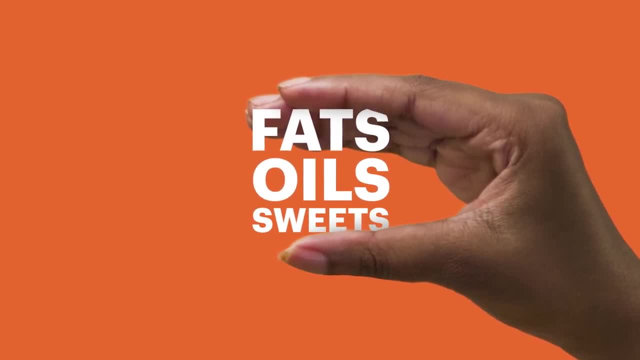 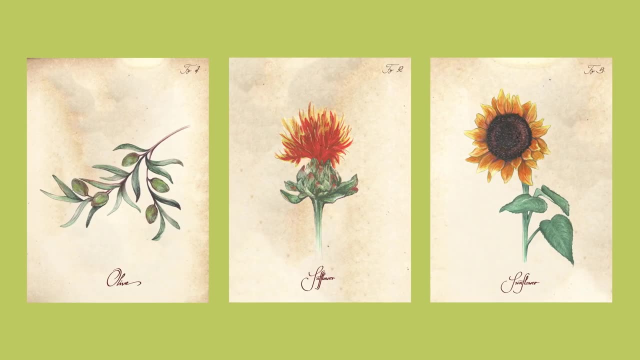 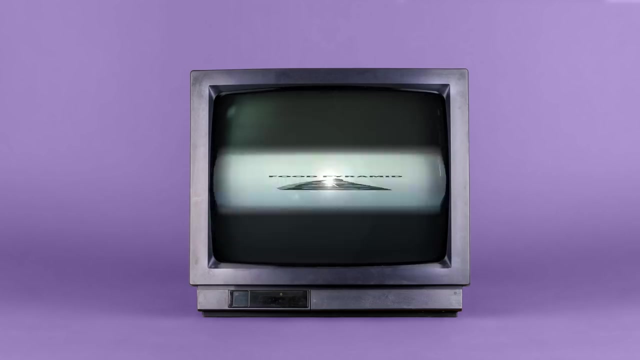 were to be used only sparingly. But some plant oils aren't bad for you. In fact. olive, safflower and sunflower oil are monosaturated fats that can actually help lower cholesterol. By 2000, critics began labeling the Food Pyramid misleading, inaccurate and confusing. 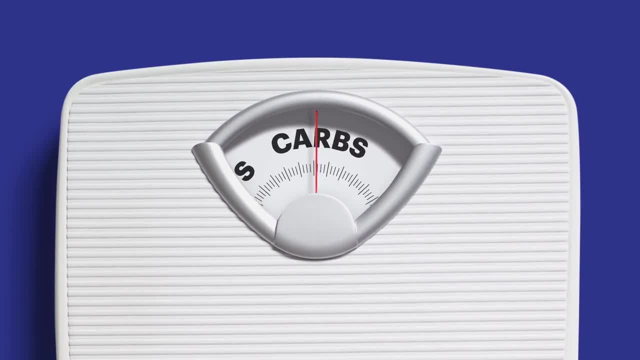 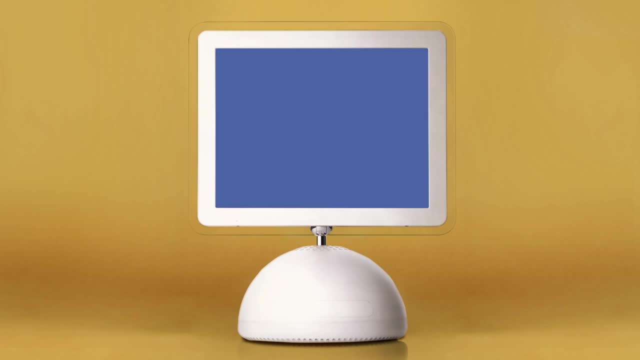 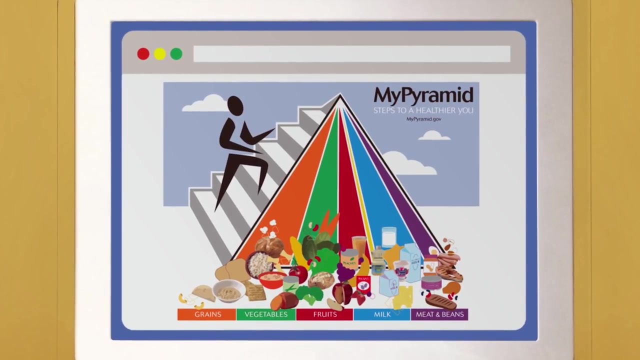 The emphasis on limiting fats, along with carbo-loading, sent a potentially harmful message to a nation struggling with rising childhood obesity rates. By 2005, health class had a new Food Pyramid featuring vertical bands of color with no text, But the new design caused even more confusion and controversy. 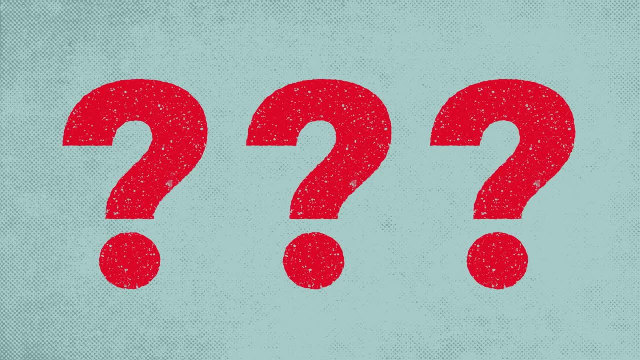 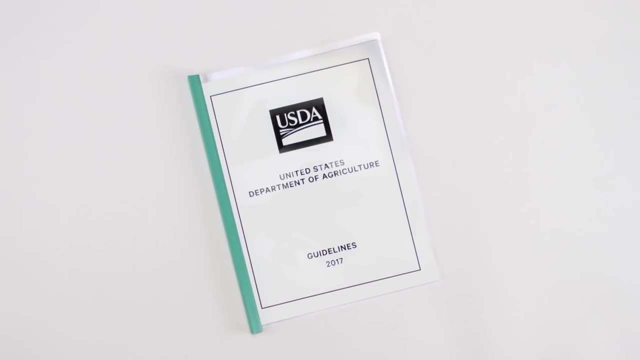 Why couldn't they get it right? The government agency that created these guidelines is the US Department of Agriculture, whose very purpose is to promote the food industry. Even though states design their own curriculum, they still use the guidelines set by the federal. 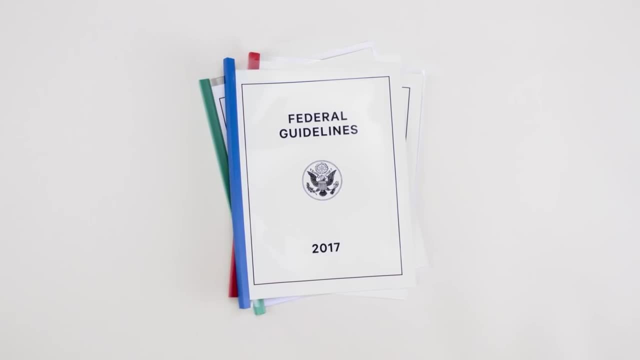 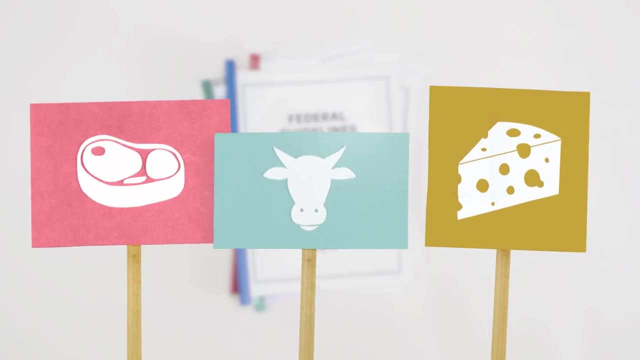 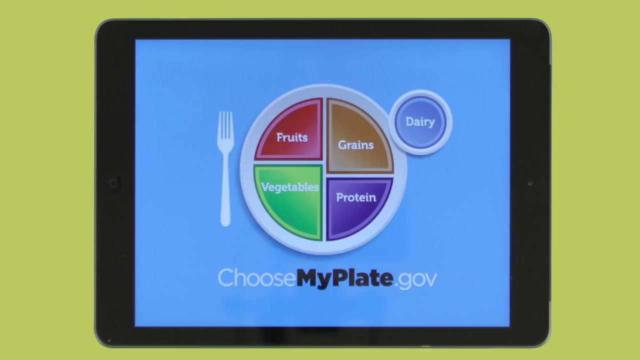 government. Some leading nutrition experts say food manufacturers, food producers and special industry groups like the meat and dairy lobby have influence in shaping recommendations. By 2011,, many health classes ditched the Pyramid design altogether and replaced it with MyPlate, an even simpler visual dietary guide. 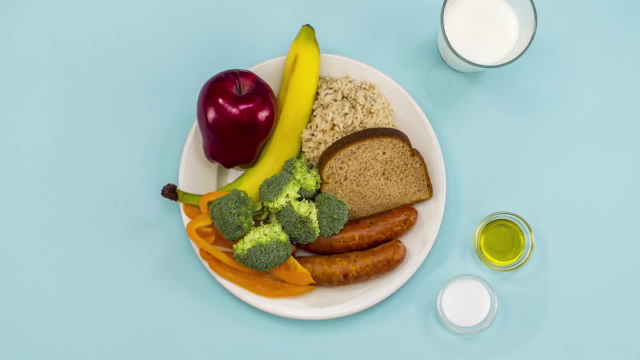 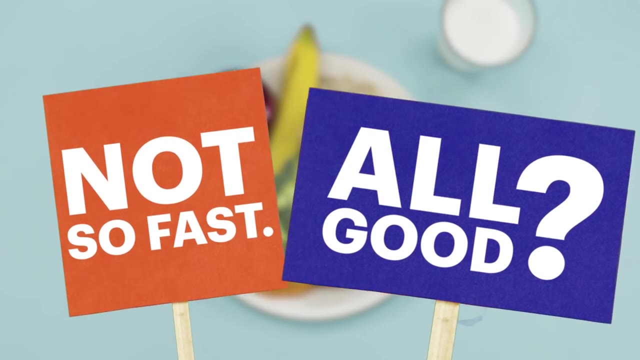 Half the plate is filled with fruits and veggies, while dairy is pushed to the side. Oil and sweets have totally vanished. So we're good now right, Not so fast. Today, experts still argue about the guidelines. How far back are we? New research is constantly shifting our direction and new possibilities are